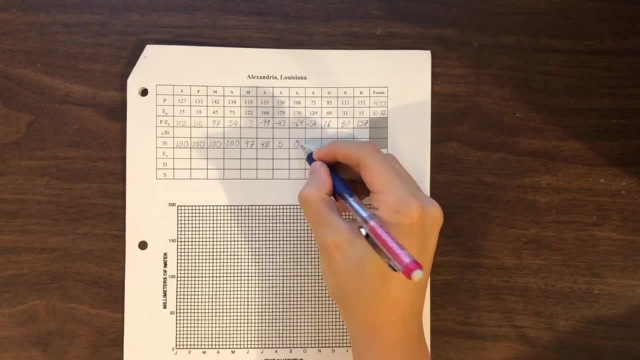 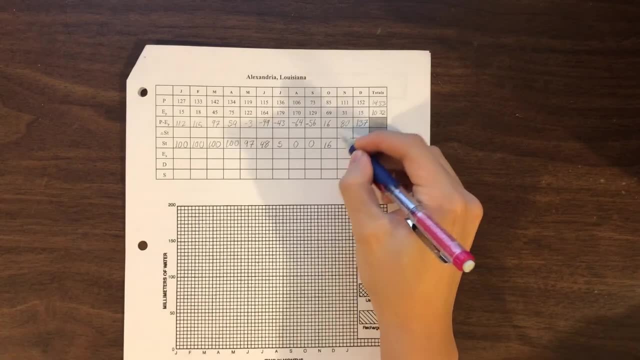 storage levels off at 0. So this just goes up to 0.. Now negative 56 goes to 0. again 16 will we're adding to 0. So this is 16, add that This is 96.. And here: 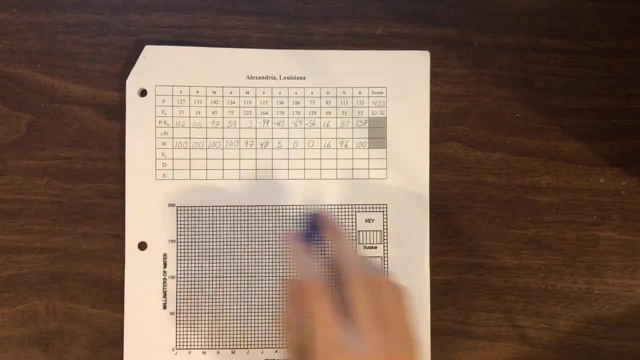 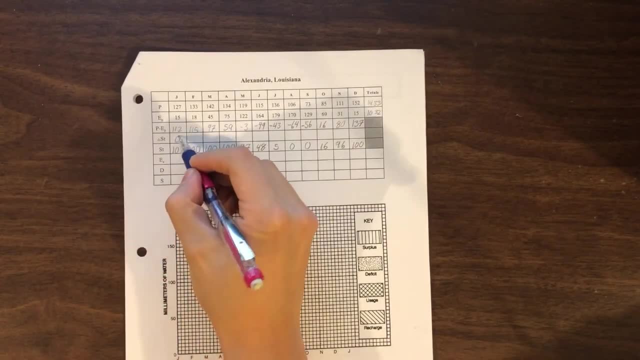 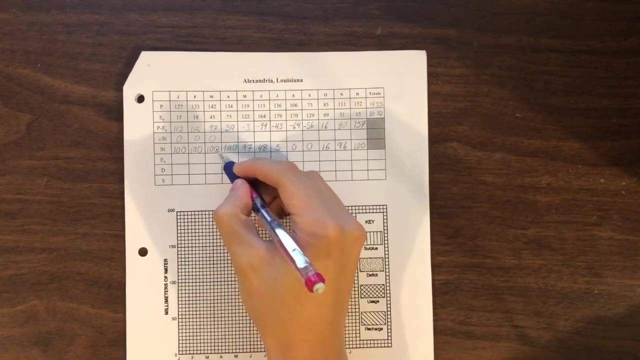 well, it caps out at 100. So it goes back to 100. Like that, Now, using this row, we can figure out what the delta storage is. So now we're going from 100 to 100. That's 0, 100 to 100, that's 0, 100 to 100, again, that's 0, 100 to 100, 0, 100 to 100, 0,. 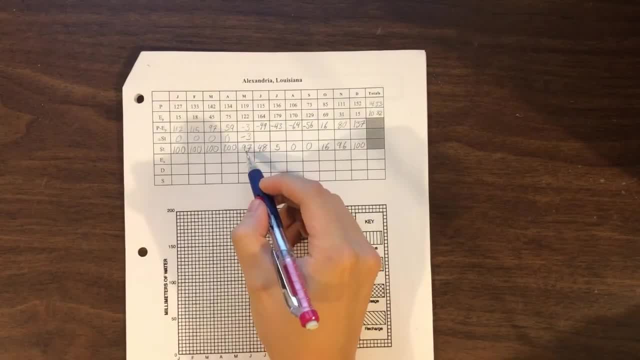 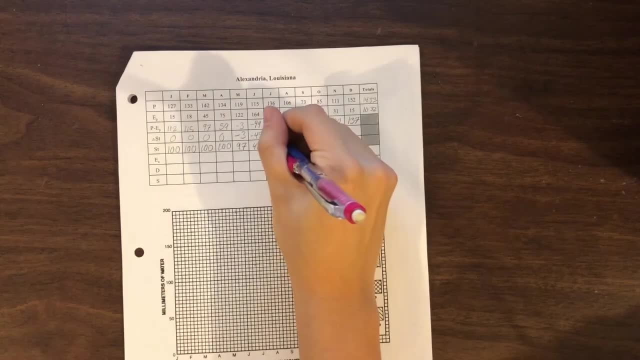 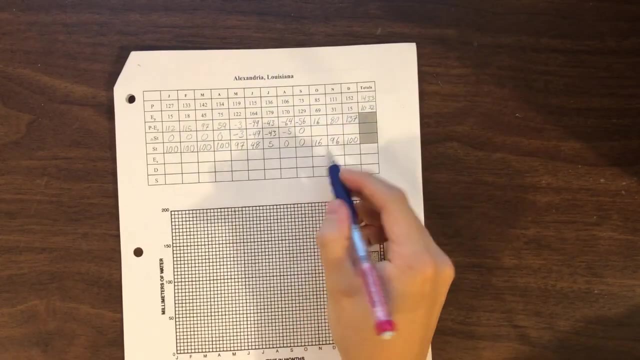 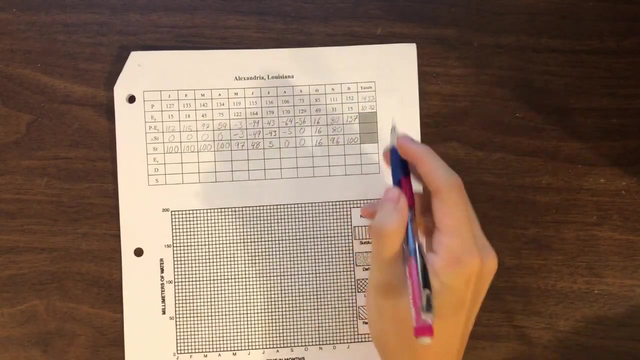 100 to 97, that's negative. 3, 97 to 49,, that's 48, that's negative. 49, 48 to 5, that's negative. 43, 5 to 0, that's negative. 5, 0 to 0, that's 0, that's addition. so 16還cake. 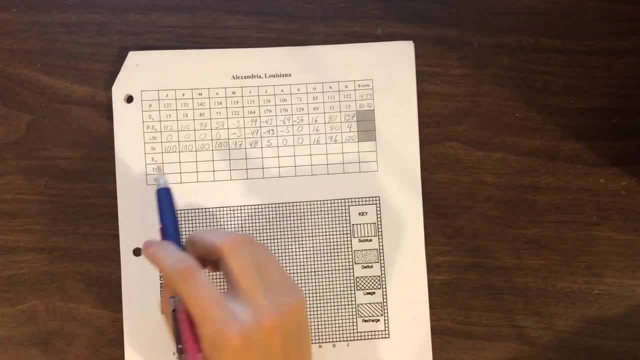 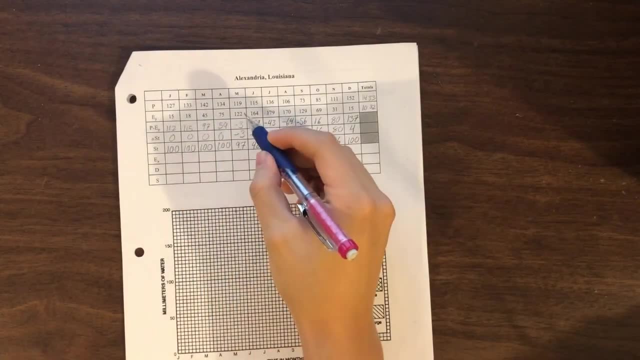 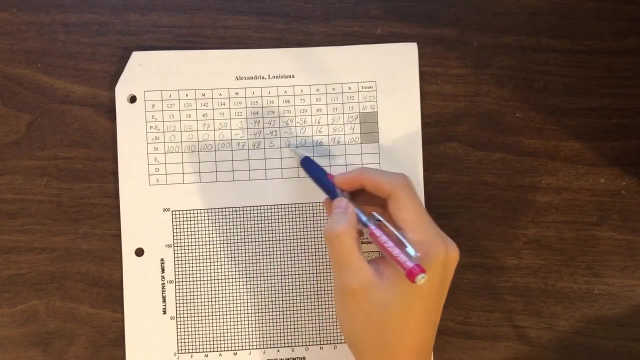 So now we've gotten that we can go on to the actual evaporation. To get the actual evaporation, what we do is we simply take the predicted evaporation and subtract stuff off if the storage is not enough, like, for example, around here. so, starting off, we 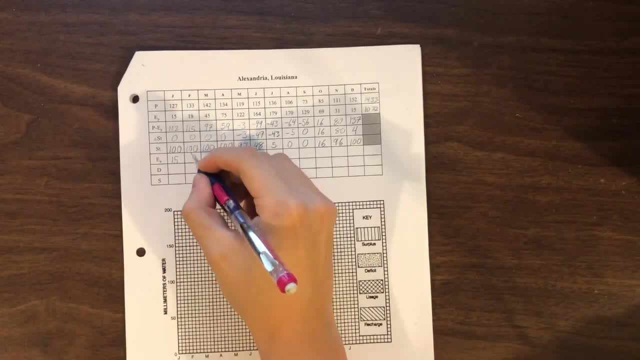 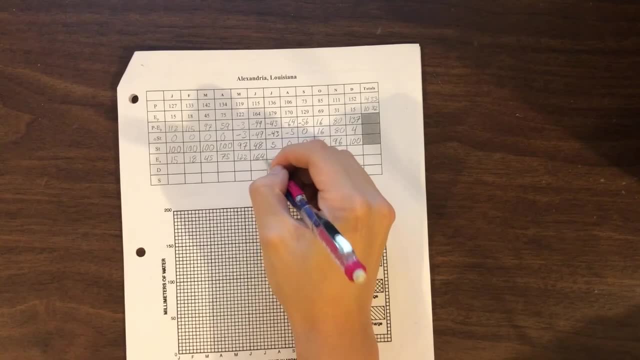 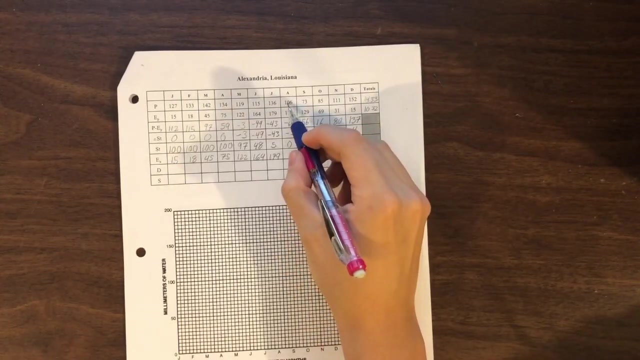 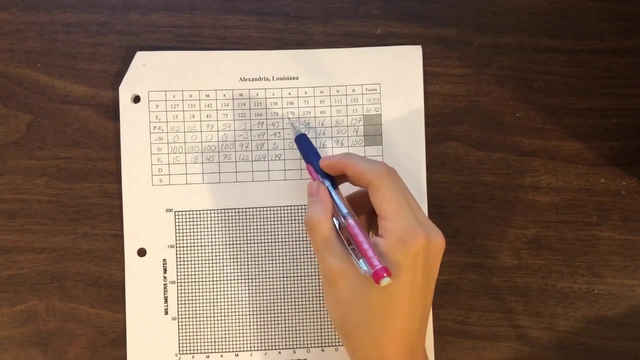 can just copy down the uh predicted evaporation: 45, 75, 122, 164, 179. all right, so now we've gotten to our first zero and starting off we see we have 106 precipitation and one on seven zero uh evaporation. well, you can't evaporate more water than you have, so you can only evaporate. 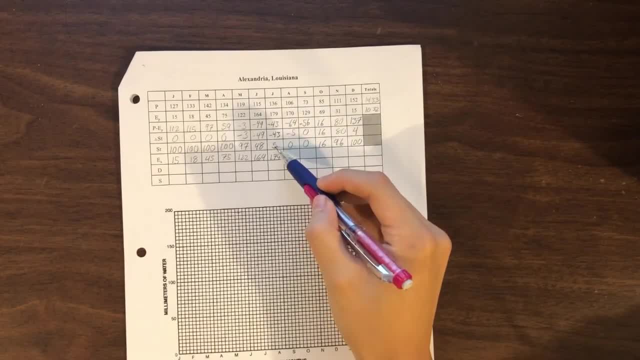 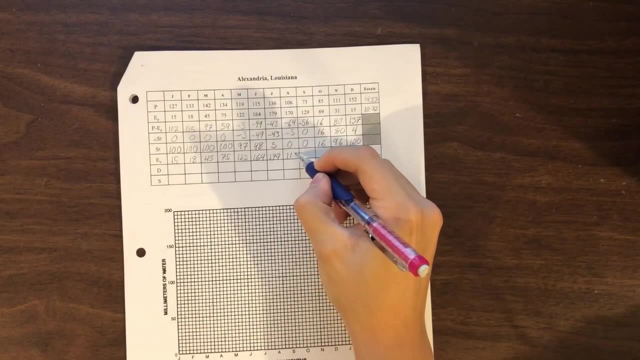 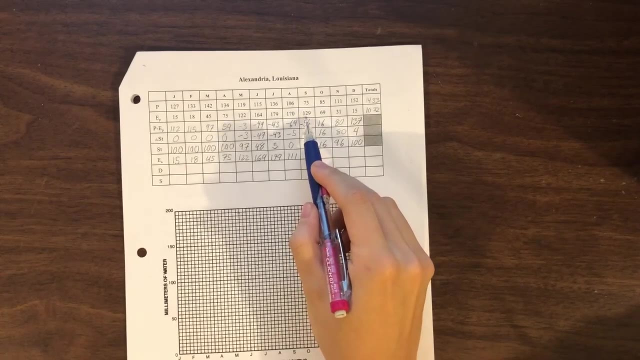 106 of the precipitation plus five from the storage over here. thus the actual precipitation is 106 plus five, or one one uh one. so here we have the same problem. uh, the precipitation is simply not enough and it's lesser than the evaporation, and there's nothing in storage. so that means that 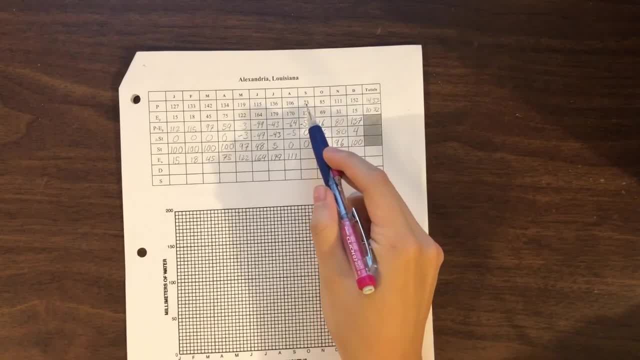 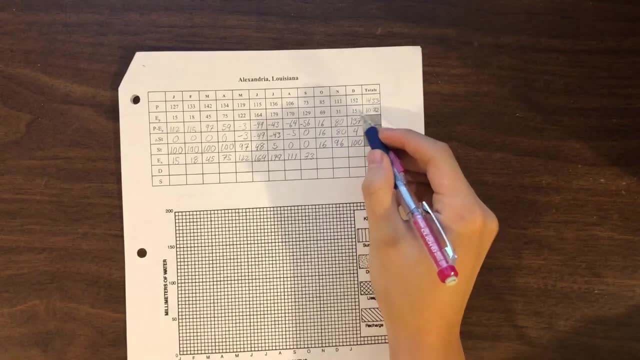 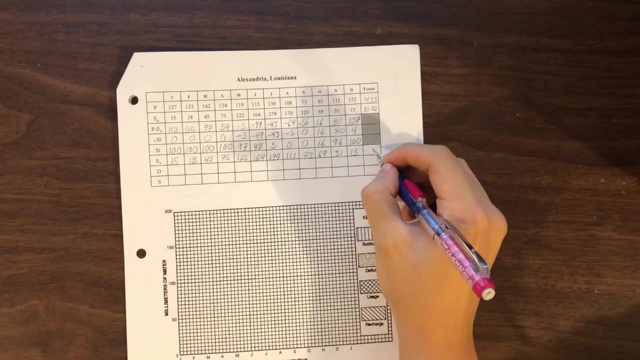 we can only take what precipitation has fallen to evaporate. thus the actual evaporation is only 73.. now we're going here, we're: this is adding, this is all less, so we can just copy it down again: 69, 31, 15, and then we will find our total. 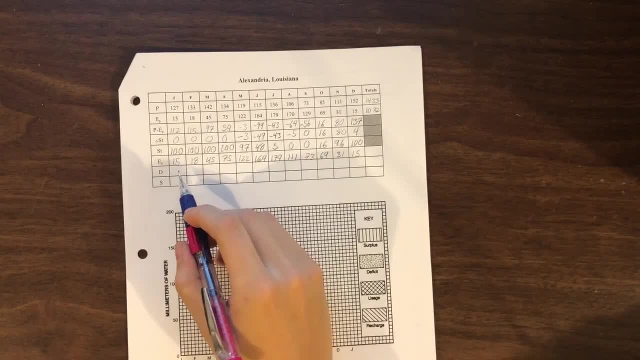 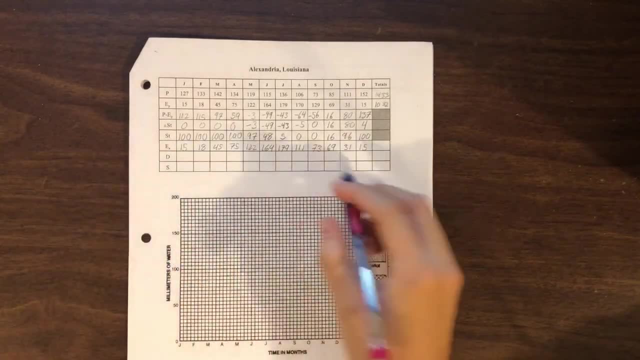 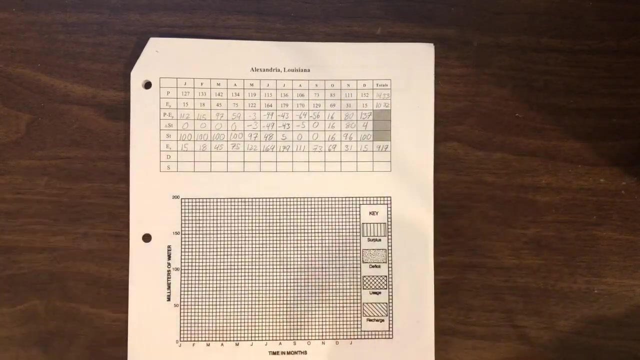 which i will do later. so now, using my amazing math skills and totally not a calculator, i've calculated the total of it. this actual evaporation is nine one seven. you know these numbers are actually pretty useless, but we'll fill them in anyway. so now we go on to 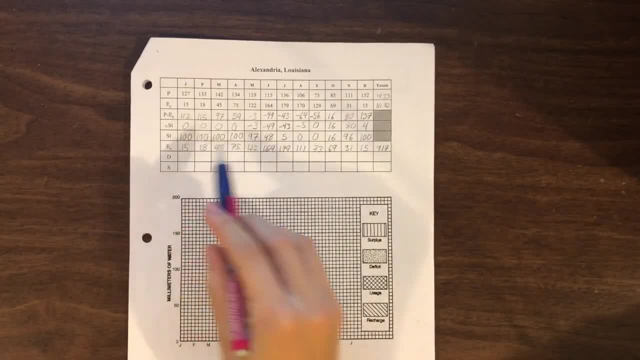 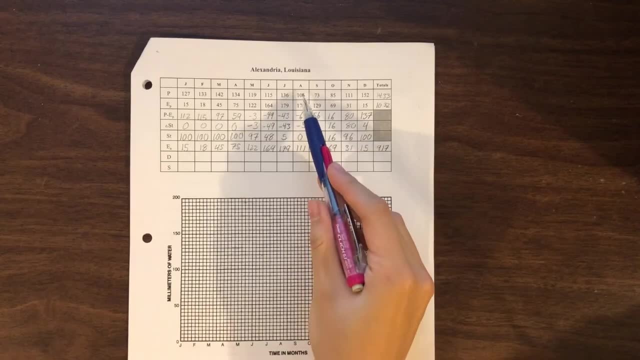 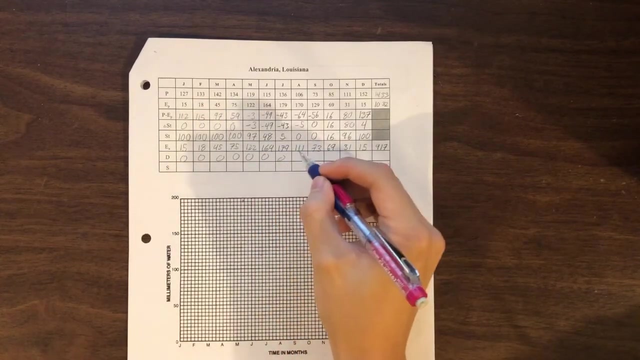 deficit. now, deficit only occurs when the storage is zero and we have to take out and, uh, there is more evaporation than there's precipitation, for example in this column. for the rest of the time it's all zero. so here, zero, zero, zero, zero, zero, zero, zero. now here we see that, uh, storage we're. 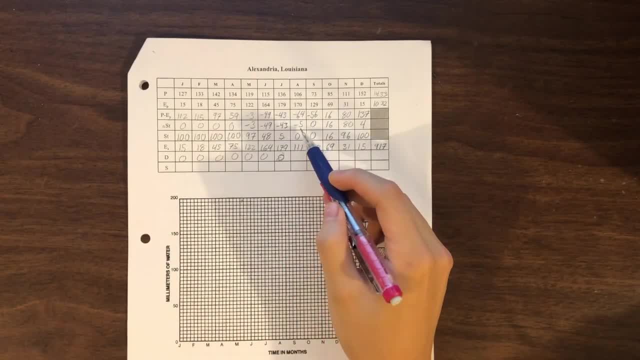 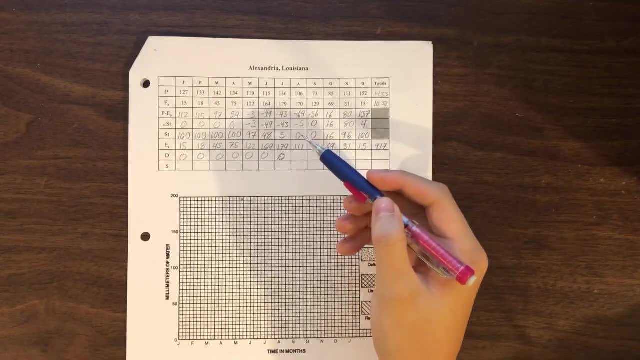 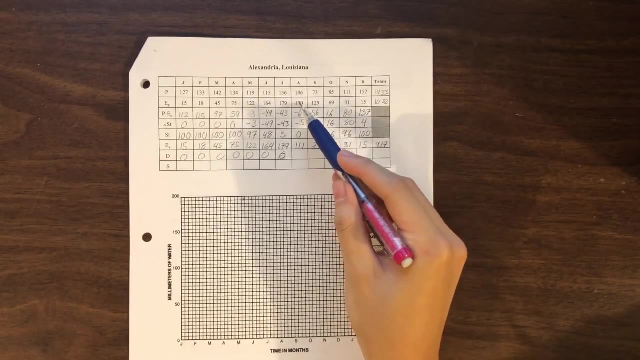 evaporating uh more than we can uh actually we have in storage and we have from precipitation. so, however much more, that is then uh how much storage there is, that is our uh deficit. so here we have 170 minus uh 106, that's we have a 64 deficit, plus there's still five in storage. so we take that away. so therefore, 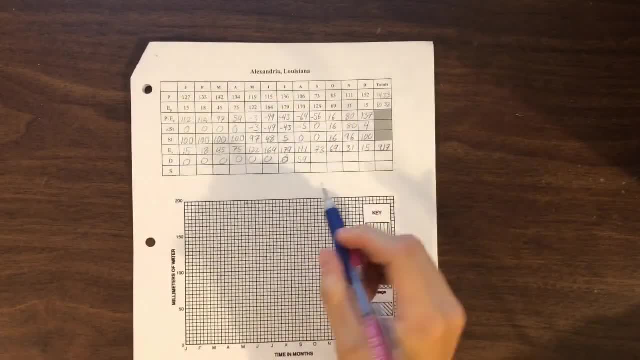 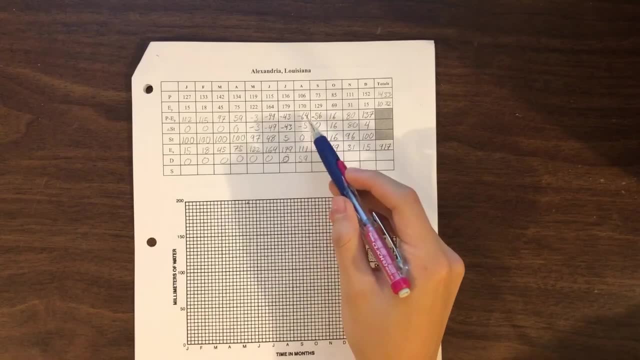 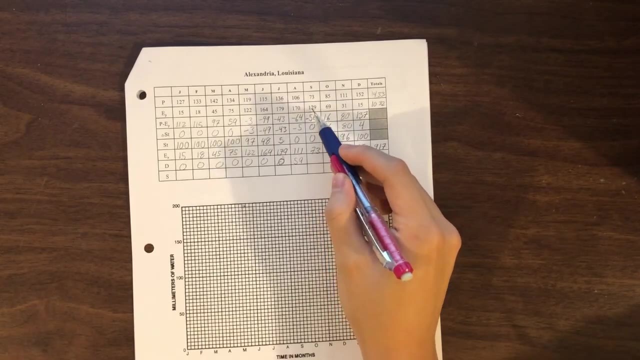 or there is a 59, uh, unit deficit here because we're trying to take away. we have to take away a 64 from the storage, but there's only five to take away. thus there's 59 that we take away from zero. make sense, good, all right. so now we have go here where the difference is negative- 56, and there's 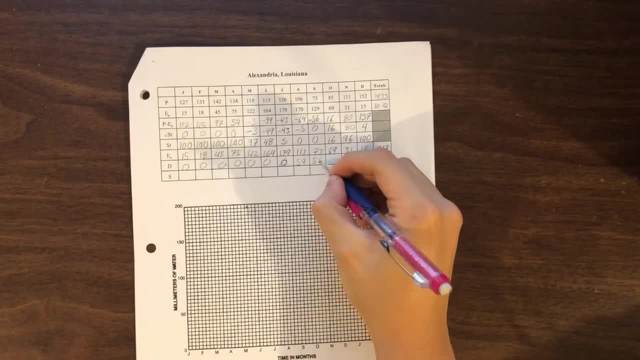 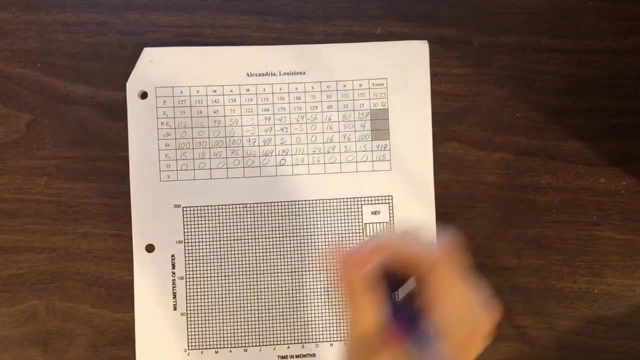 nothing to take away. so it's just the deficit of 56, and here we're adding and adding. so zero, zero, zero. at least the other, that is 115.. so now we go to our surplus. this only occurs when the storage is a hundred and we are adding more water to the storage. 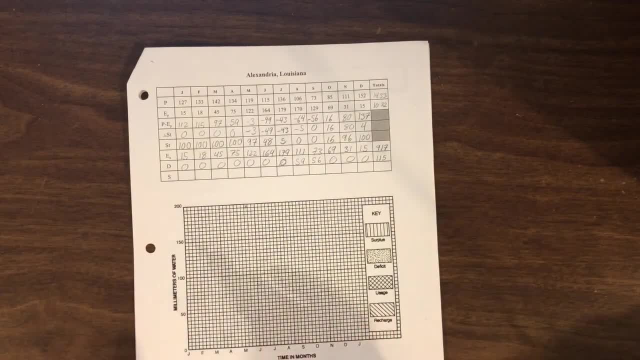 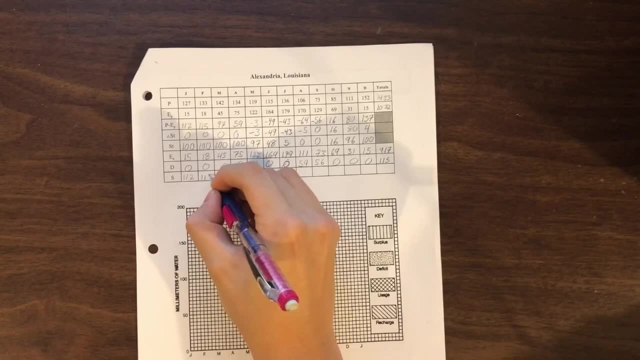 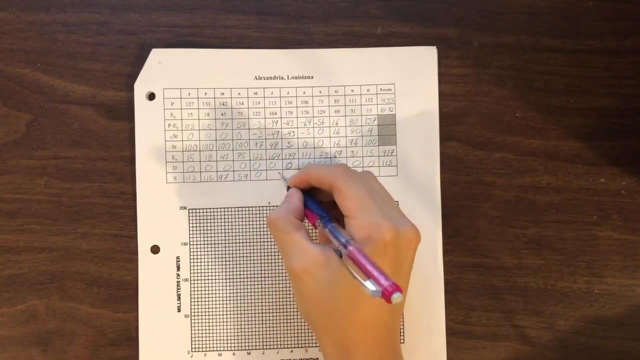 this results in runoff which just goes away from the storage and we'll call surplus. so here we're adding 112, so that's 112 surplus, here 115, here 97 and here 59 and here's uh taking away. so we don't worry about those, those are all zero. 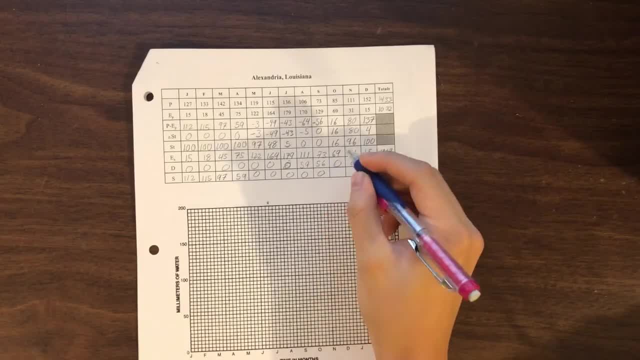 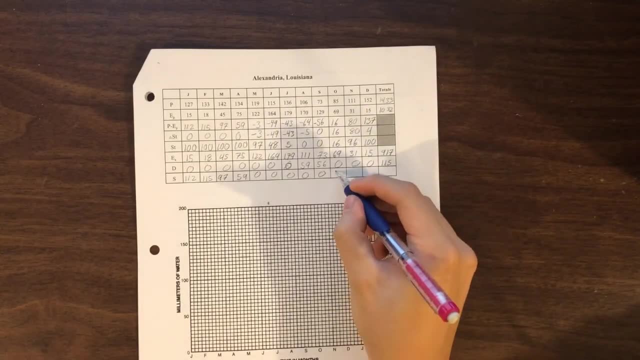 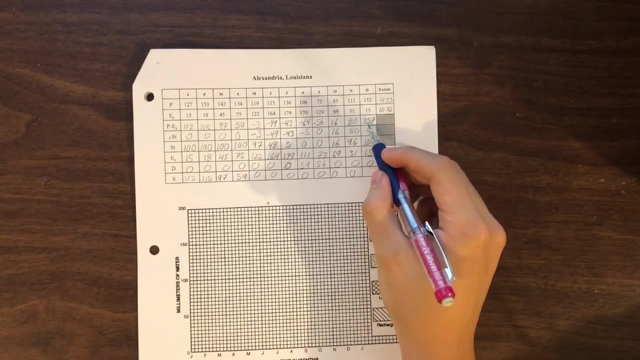 for obvious reasons, you aren't adding anything if you're taking away. and now we're at 16, well, storage isn't full, so this all goes into storage. now, if it goes off, into runoff. so therefore, the yeah, same thing. it's still filling up storage. so zero. now, here we have, we're adding 137. 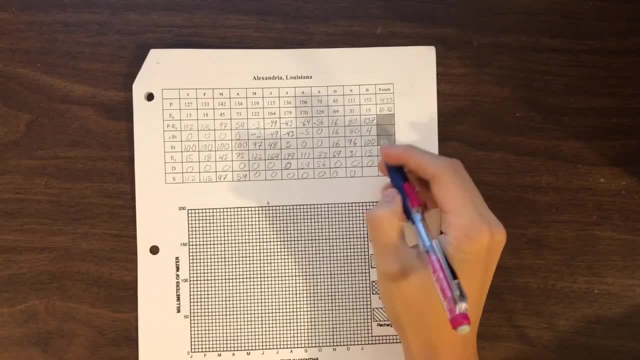 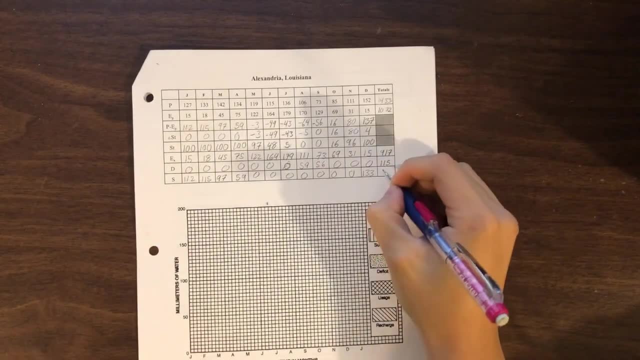 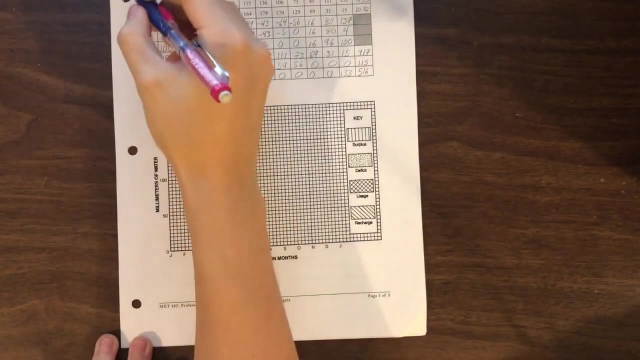 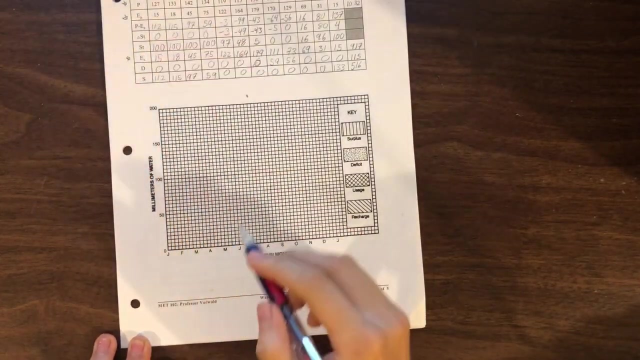 and four of that goes into filling up storage, the other 133 that goes into surplus. so now our total is 516.. so now let's go on to the graph. uh, we are required to graph the precipitation, uh, predicted evaporation and actual evaporation on this uh plot right here. so 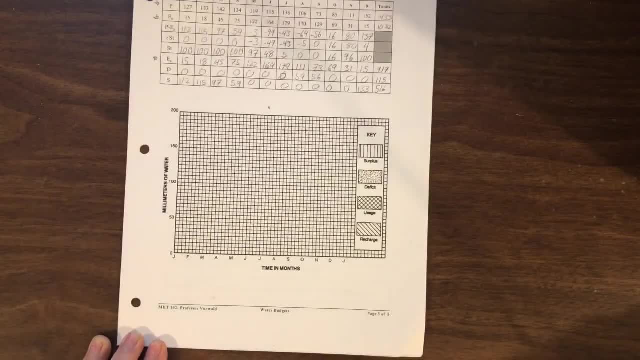 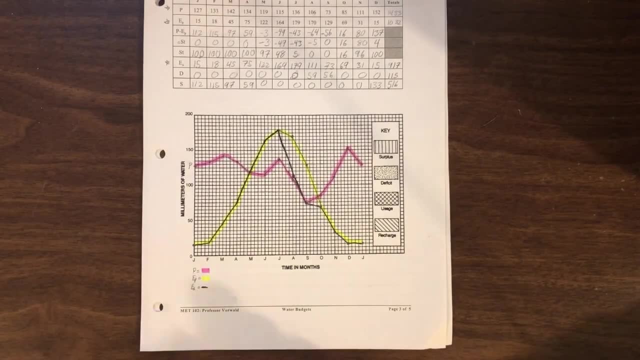 i will go and plot those and then we'll come back later to uh fill in the gaps. all right now. you see i have graphed the uh three values. right here we have precipitation in pink, the predicted evaporation in yellow and the actual evaporation in a sharpie black right here. 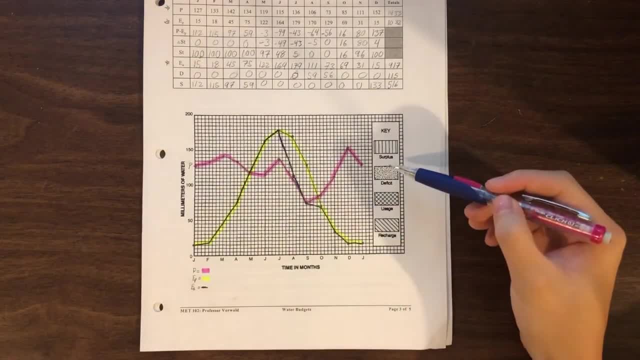 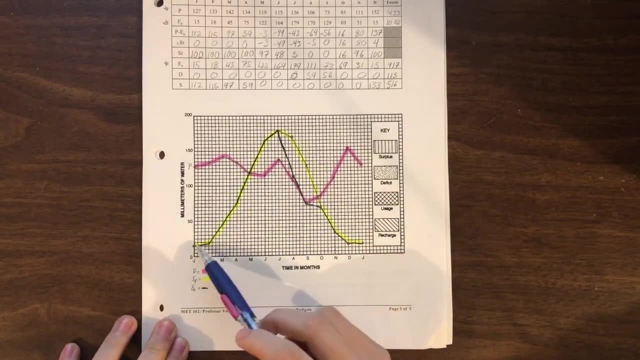 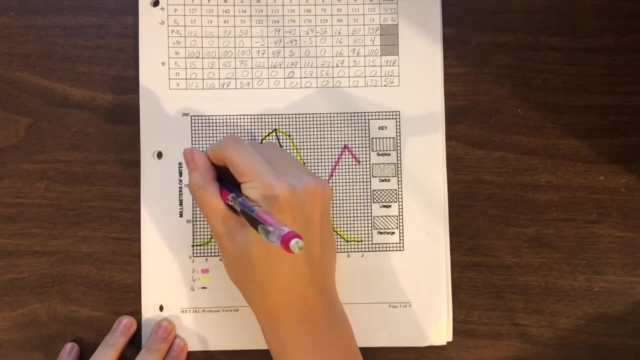 all right. so now we have to label the areas between these with surplus, deficit, usage and recharge. well, first of all, all here, all of this is beginning with storage at 100, so it's all surplus. so we can simply just draw some lines here to indicate that it is surplus. 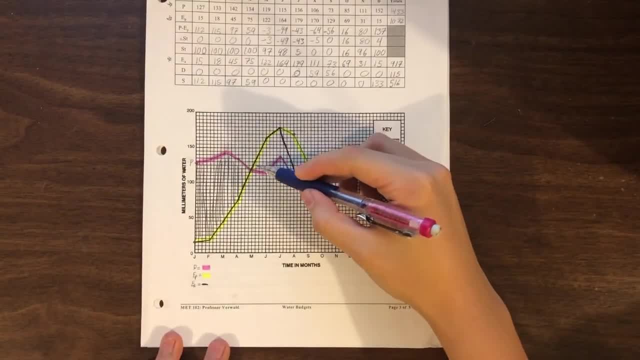 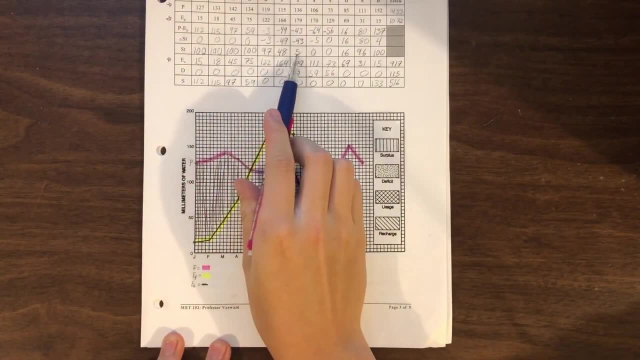 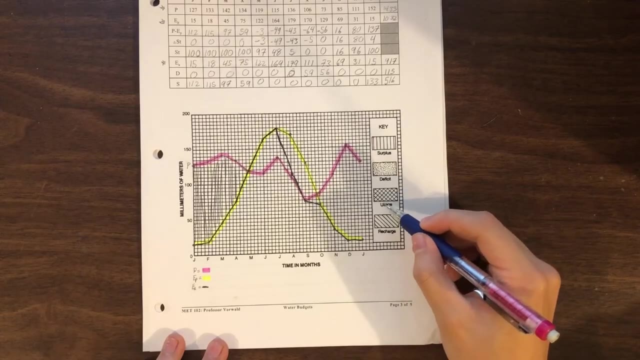 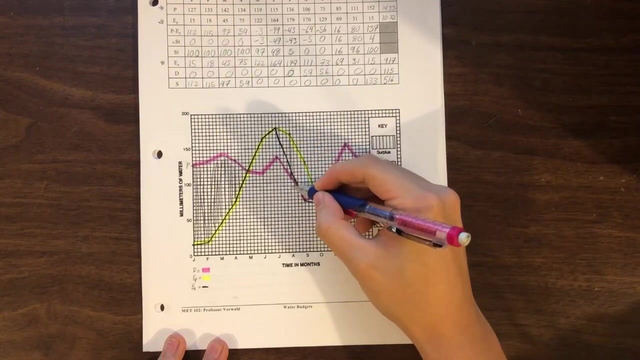 all right now that none of that is good of that is done. here is where we are taking water away from uh the storage. as you can see here, the storage is decreasing in these three months. right here, this is where we are, are using the uh water right here, so it is usage. this goes up on to uh april, in which case we end up uh. 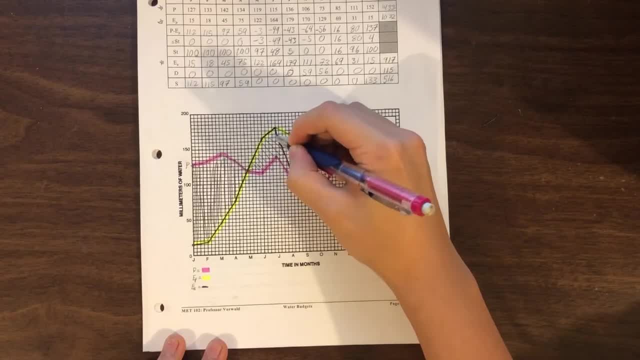 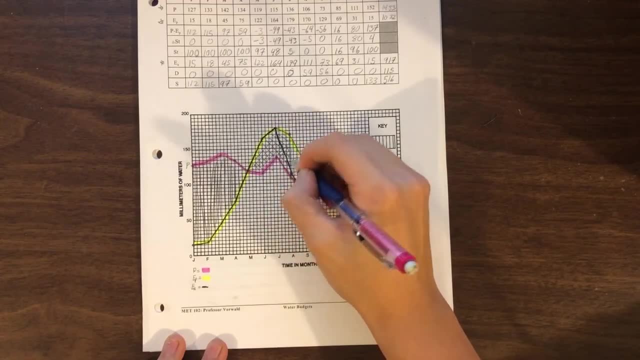 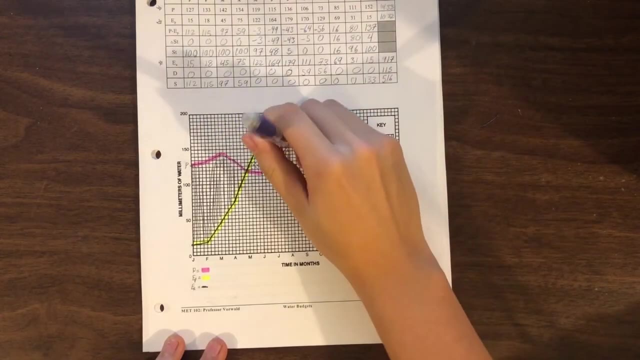 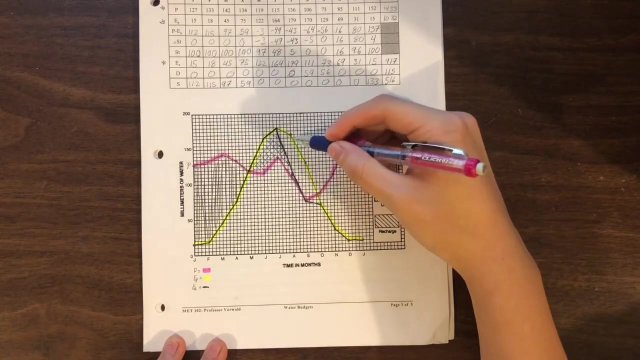 actually running out of water in the storage and becomes deficit. so we shall fill in this area here with this to represent usage. so then here, here is where we have a deficit. actually, wait, here would be deficit too. so basically, here is where we would have a deficit. 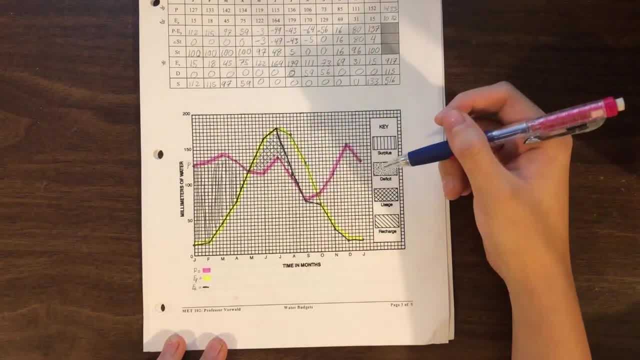 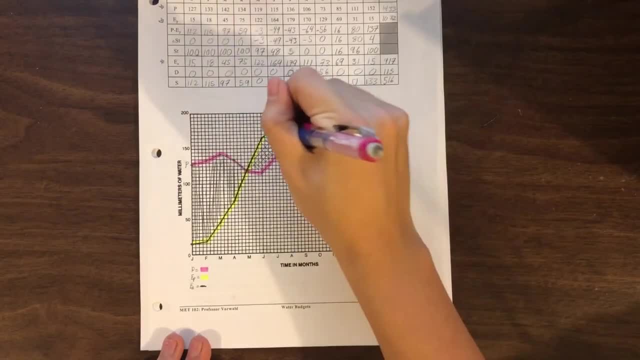 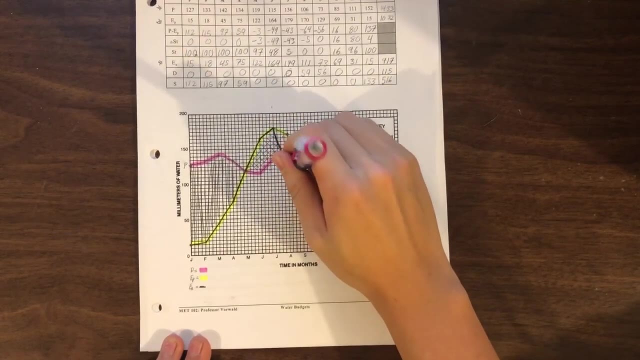 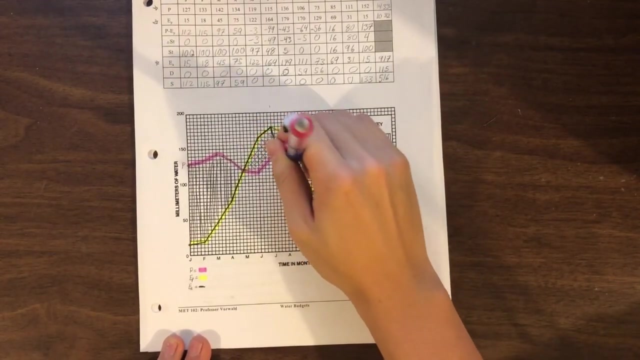 this would be all the water that would be evaporated but cannot be evaporated due to the fan and that there is simply no water in storage. so deficit here is labeled as dot. so we just this is really bad for my pencil. so yeah, basically just fill that place up to the heck worth. uh, dots.